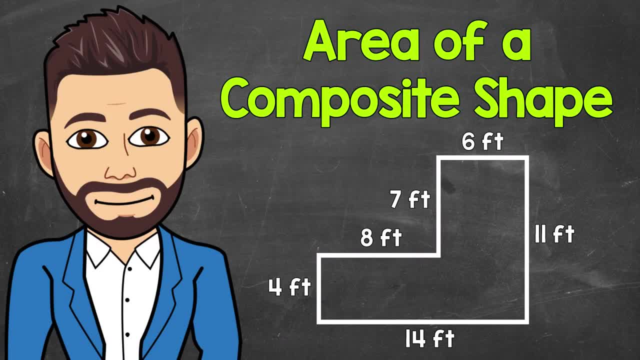 Welcome to Math with Mr J. In this video I'm going to cover how to find the area of a composite shape. Now remember: area is the amount of space or surface inside of a shape, So how much space or surface something covers? 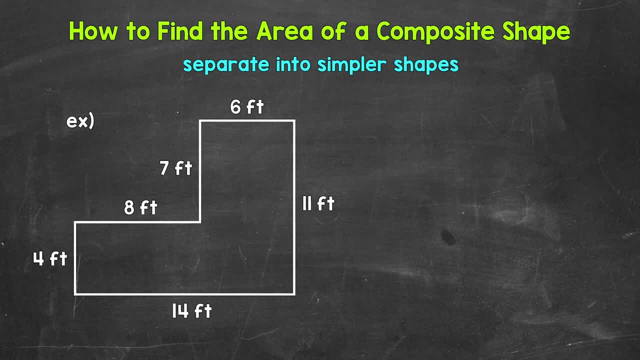 When we find the area of composite shapes, we can separate the shape into simpler shapes. We find the area of those shapes and then add them together to find the total area. Let's jump into our example And you'll notice we don't have a simple rectangle, square triangle or whatever the case may be. 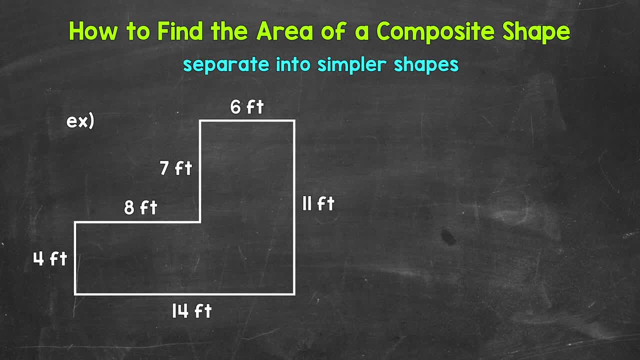 that we can easily find the area of. So let's separate this shape, or break this figure up into simpler shapes to work with. Now, there are different ways to separate this figure, but I'm going to separate it into a top and a bottom. 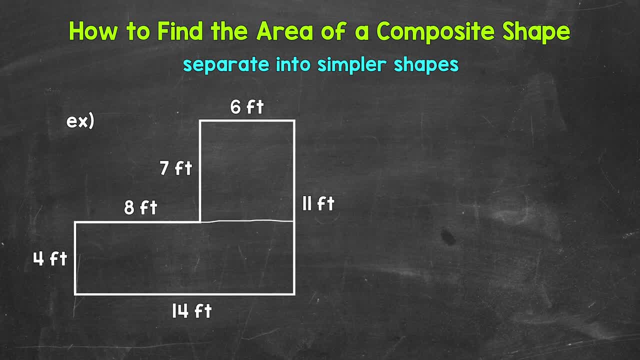 So let's separate this into a top and a bottom rectangle. Now you can also separate this into a left and a right. Either way is correct, and you will get the same total area in the end. Now let's call this shape A and this shape B. 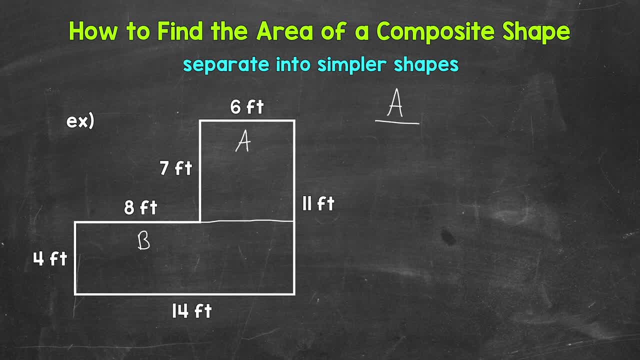 Let's start by finding the area of A, And since it is a rectangle, let's use the formula: area equals length times width. Now I'm using a cursive, L. that way it doesn't look like a 1.. Now we need to find the correct length and width for rectangle A. 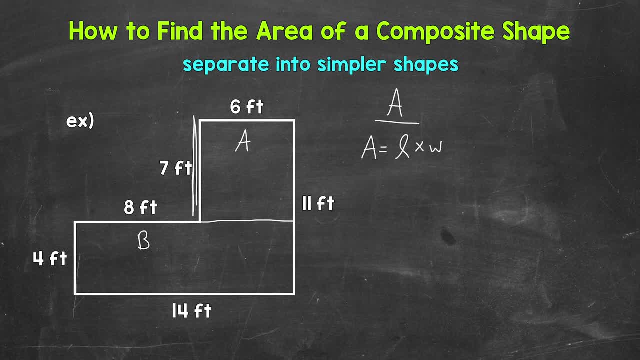 Well, this is a 7 by 6 rectangle, So let's plug those in 7 times 6.. It's very important that we pick the correct length and width. For example, we don't need this 11 feet here. 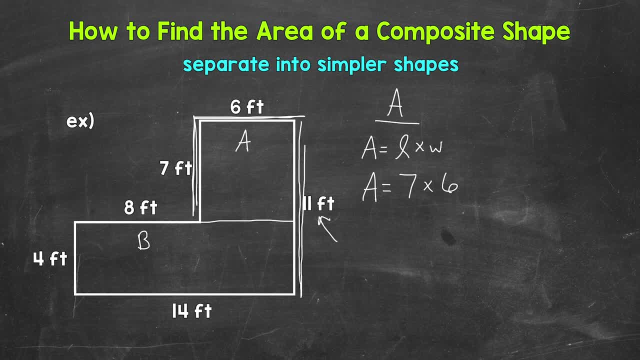 That goes all the way down here. So be careful about which side lengths you are using for calculating the area. I also want to mention: don't get too held up on which is the length and which is the width. I'm using the longer side length for the length to keep it consistent. 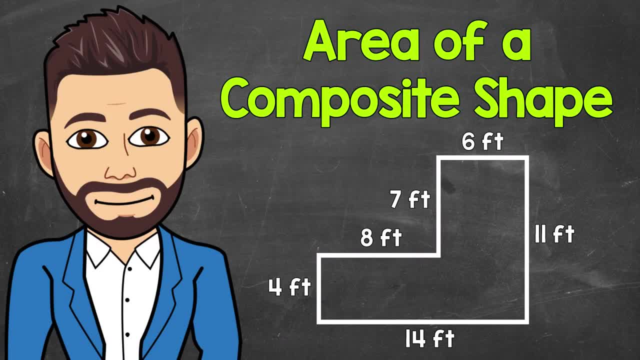 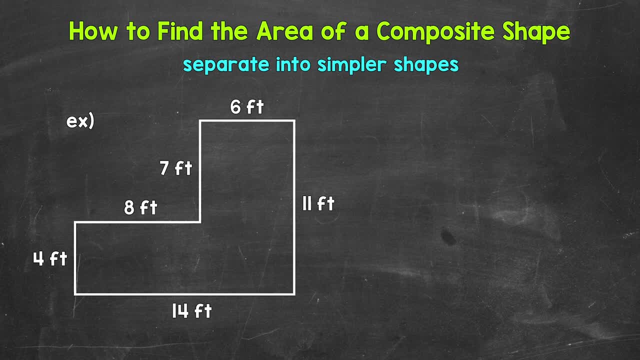 Welcome to Math with Mr J. In this video I'm going to cover how to find the area of a composite shape. Now remember: area is the amount of space or surface inside of a shape, So how much space or surface something covers? 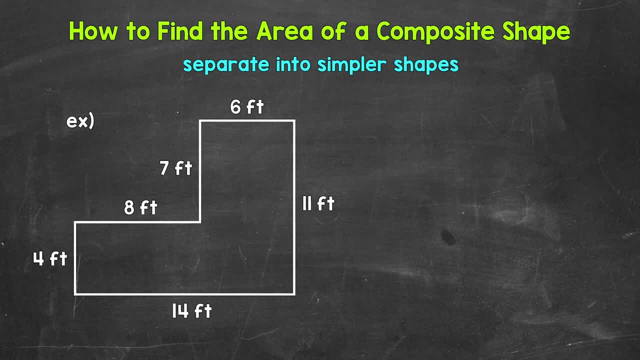 When we find the area of composite shapes, we can separate the shape into simpler shapes. We find the area of those shapes and then add them together to find the total area. Let's jump into our example And you'll notice we don't have a simple rectangle, square triangle or whatever the case may be. 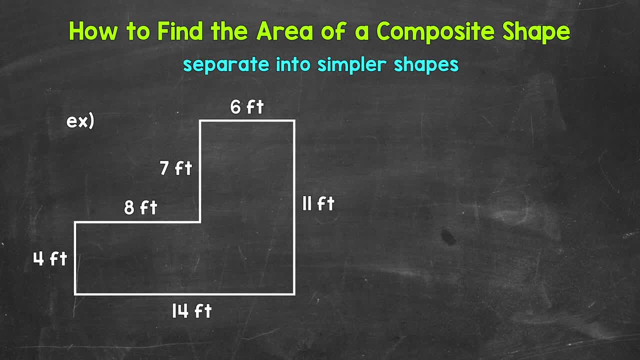 that we can easily find the area of. So let's separate this shape, or break this figure up into simpler shapes to work with. Now, there are different ways to separate this figure, but I'm going to separate it into a top and a bottom. 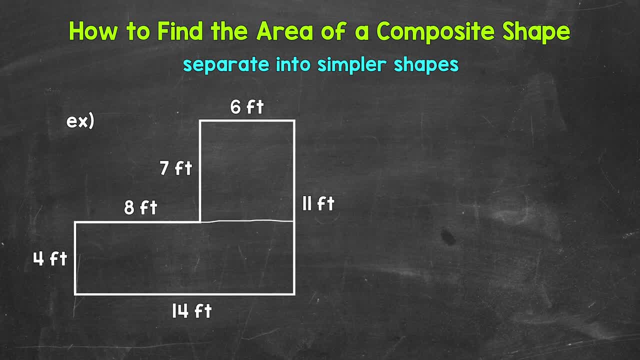 So let's separate this into a top and a bottom rectangle. Now you can also separate this into a left and a right. Either way is correct, and you will get the same total area in the end. Now let's call this shape A and this shape B. 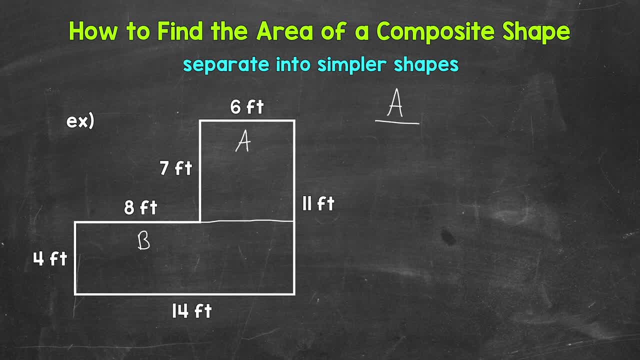 Let's start by finding the area of A, And since it is a rectangle, let's use the formula: area equals length times width. Now I'm using a cursive, L. that way it doesn't look like a 1.. Now we need to find the correct length and width for rectangle A. 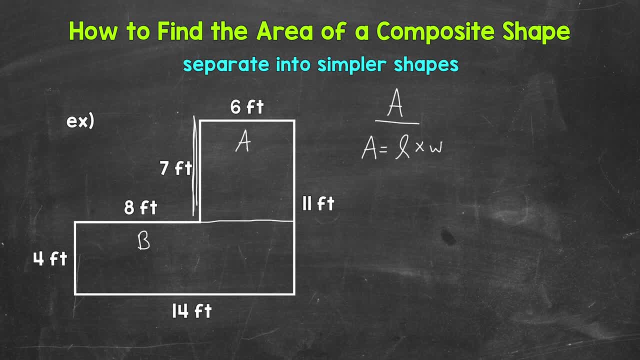 Well, this is a 7 by 6 rectangle, So let's plug those in 7 times 6.. It's very important that we pick the correct length and width For the given rectangle. For example, we don't need this 11 feet here. 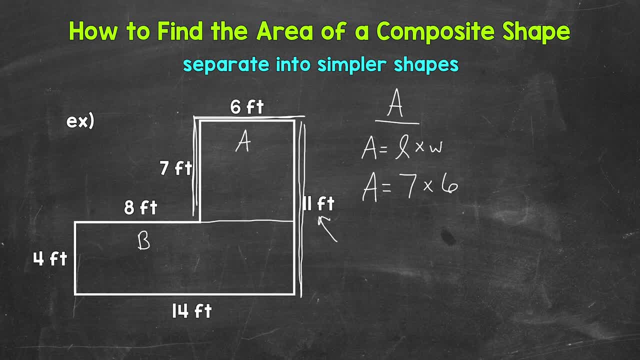 That goes all the way down here. So be careful about which side lengths you are using for calculating the area. I also want to mention: don't get too held up on which is the length and which is the width. I'm using the longer side length for the length to keep it consistent. 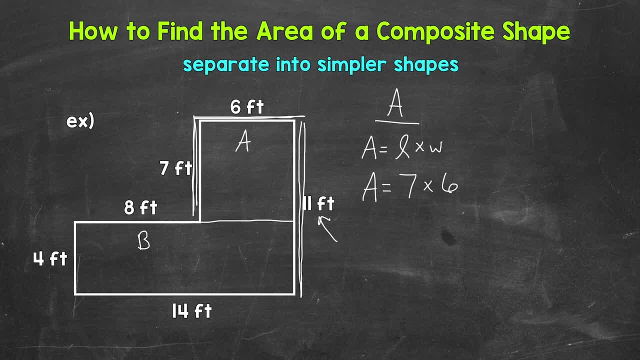 But really you're going to get the same area either way. So in my opinion, don't get too held up on which is the length and which is the width. Just make sure you are using the correct sides for calculating that area. So as far as the area for A, 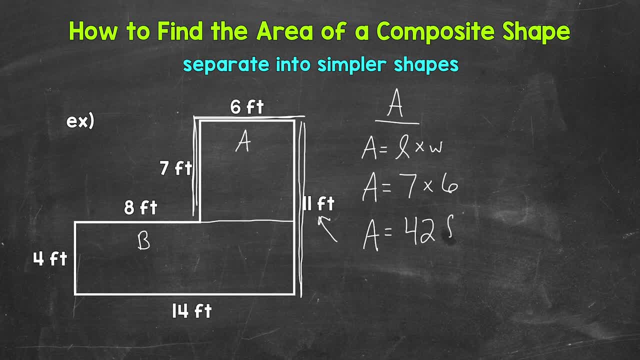 seven times six gives us 42, and this is square feet. So the area here is 42 square feet. Now we need to find the area of B, So area equals length times width. So now let's pick out the correct sides here. 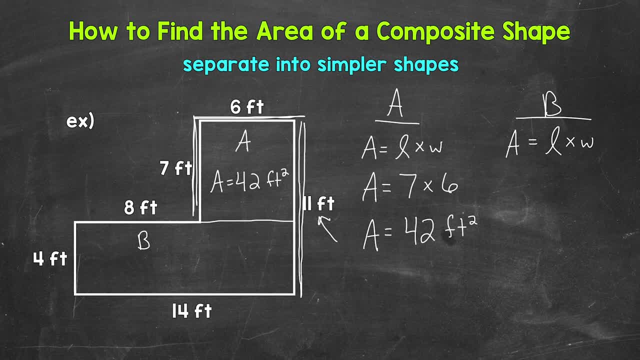 as far as what we need to calculate the area, This is a 14 by four rectangle, So 14 feet by four feet. So let's plug those in Again. I'm using the longer side length for the length, So 14 times four. 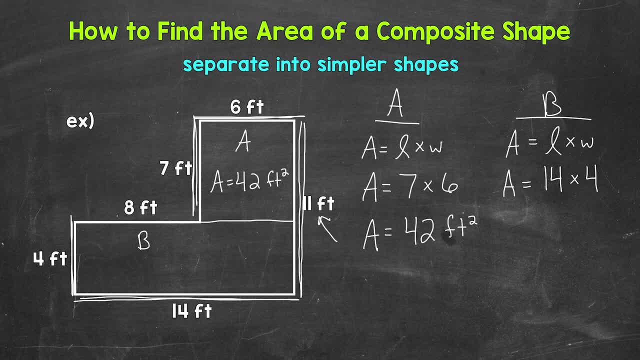 Now, before we multiply 14 times four, I do want to mention we did not need this eight feet, because that only goes to that point. We needed the 14 feet all the way across the bottom of that rectangle. So again, we need to be careful. 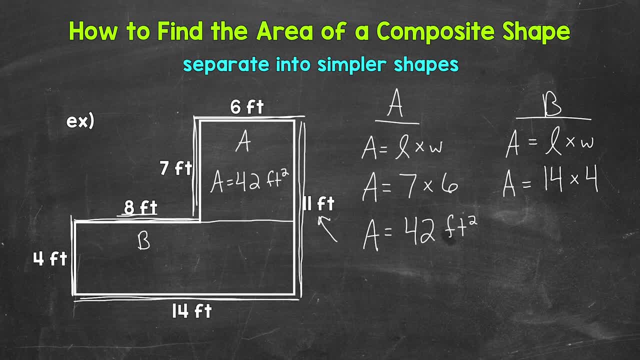 as far as which side lengths we are using. So now let's multiply 14 times four. So 14 times four equals 56. So the area of B is 56 square feet. Now we have all of the information we need to find the total area of the composite shape. 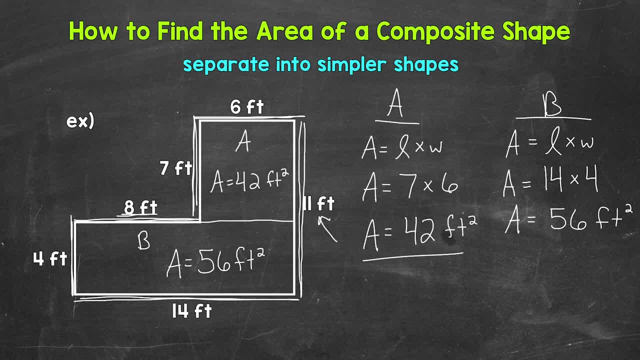 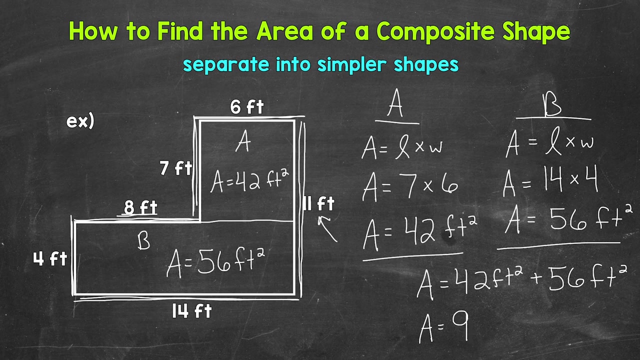 We need to add A, so 42 square feet, plus B- 56 square feet. So the total area we have 42 square feet plus 56 square feet. 42 plus 56 gives us 98 square feet And that's our final answer here. 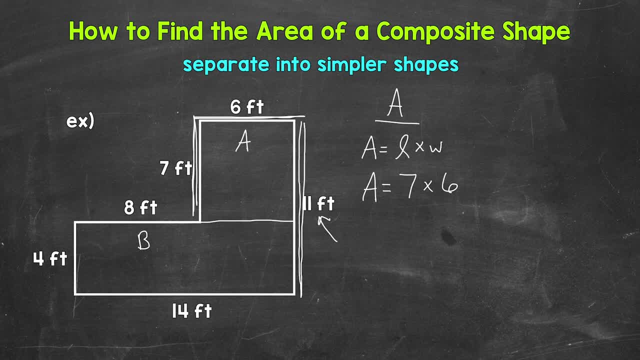 But really you're going to get the same area either way. So in my opinion, don't get too held up on which is the length and which is the width. Just make sure you are using the correct sides for calculating that area. So as far as the area for A, 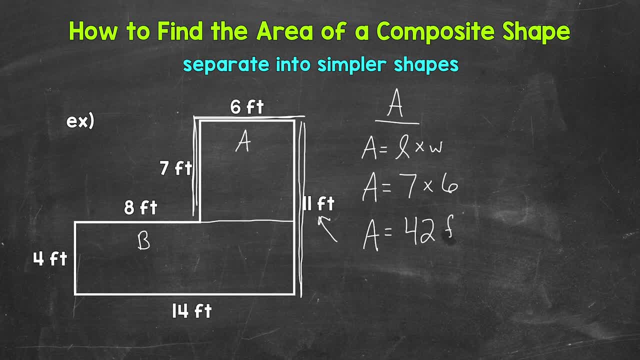 7 times 6 gives us 42. And this is square feet. So the area here is 42 square feet. Now we need to find the area of B, So area equals length times width. So now let's pick out the correct sides here. as far as what we need to calculate the area. 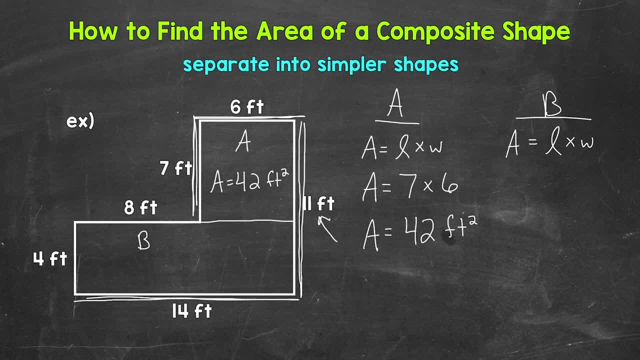 This is a 14 by 4 rectangle, So 14 feet by 4 feet. So let's plug those in Again. we're using the longer side length for the length, So 14 times 4.. Now, before we multiply 14 times 4,. 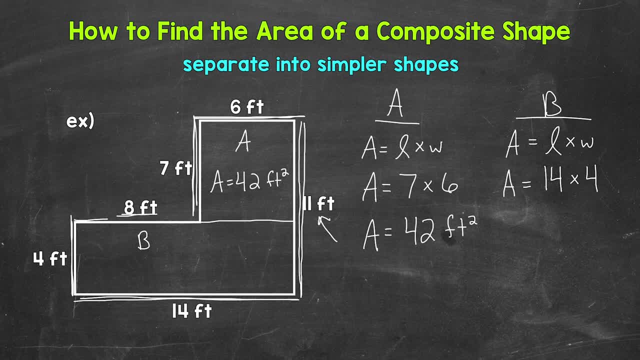 I do want to mention we did not need this 8 feet because that only goes to that point. We needed the 14 feet all the way across the bottom of that rectangle. So again, we need to be careful as far as which side lengths we are using. 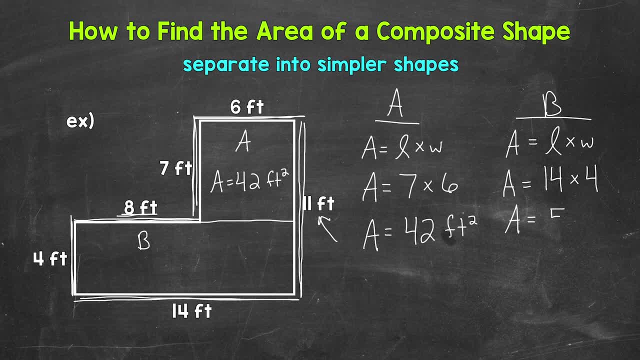 So now let's multiply 14 times 4 equals 56. So the area of B is 56 square feet. Now we have all of the information. we need to find the total area of the composite shape, We need to add A. 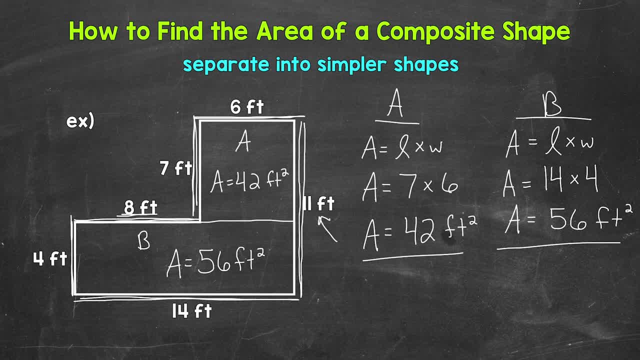 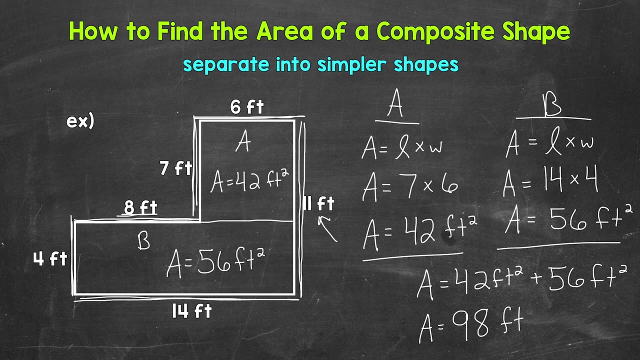 so 42 square feet plus B 56 square feet. So the total area we have 42 square feet plus 56 square feet. 42 plus 56 gives us 98 square feet And that's our final answer here, the final area of that composite shape.